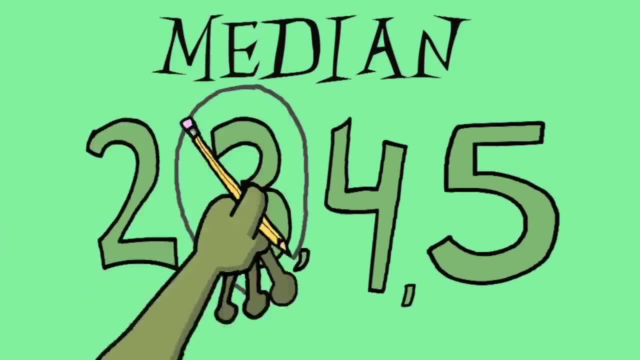 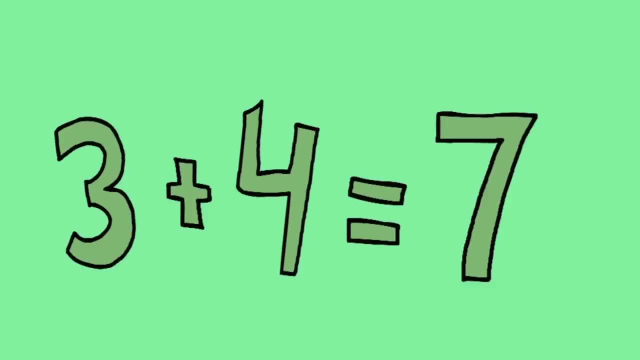 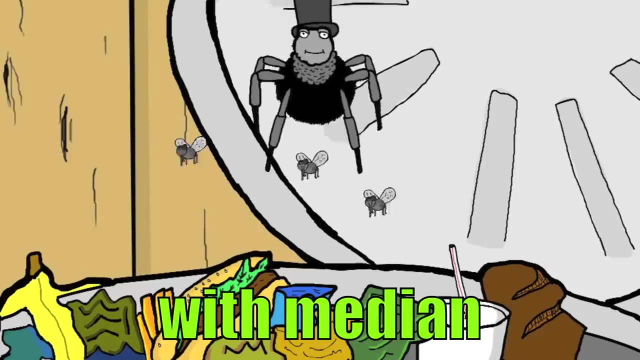 Circle the numbers And then you add the two numbers in the middle. Then add those two numbers together and divide them by two. In the middle, in the middle, in the middle for Median Circle, the number in the middle, Add and divide by two. 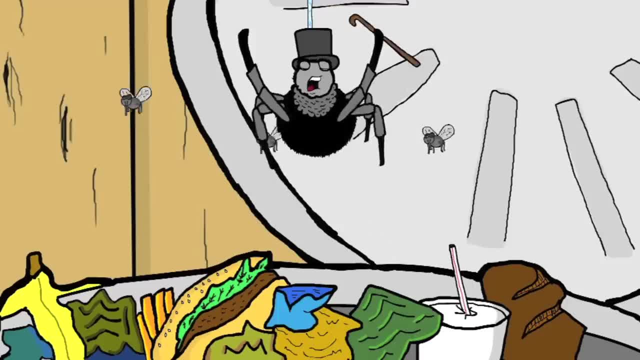 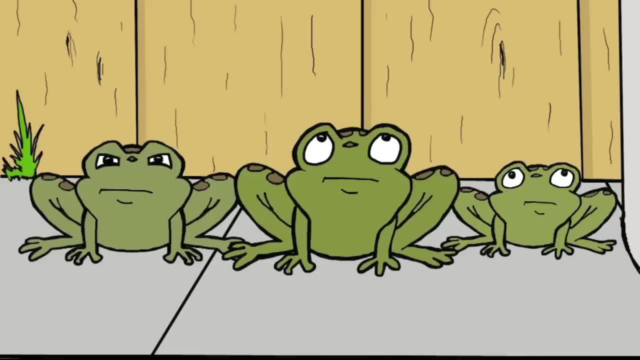 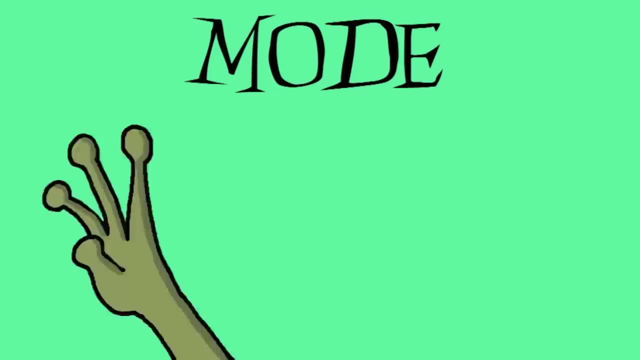 In the middle. Oh yeah, Last but not least, it's me the Mode Toad. What I do is I find the most common number the most popular, like me, of course. First I make up my list from least to greatest. 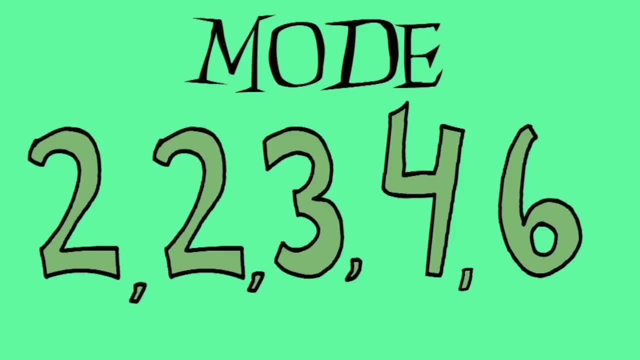 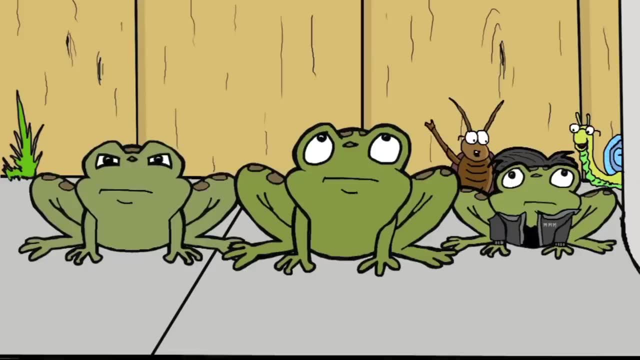 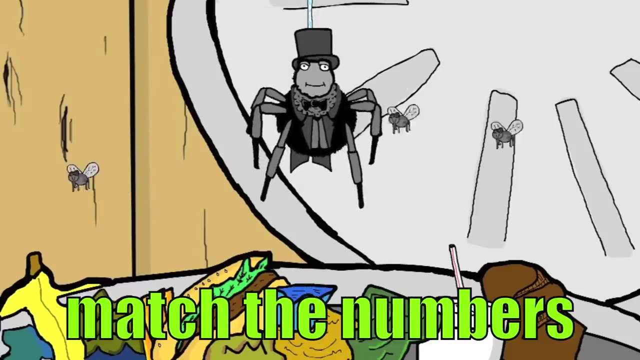 Then I see if there are any numbers that are the same. The most numbers that are the same are the Mode, like me, the most popular. Put all the numbers in that line, Small to big. you're doing fine: Match the numbers that are the same. 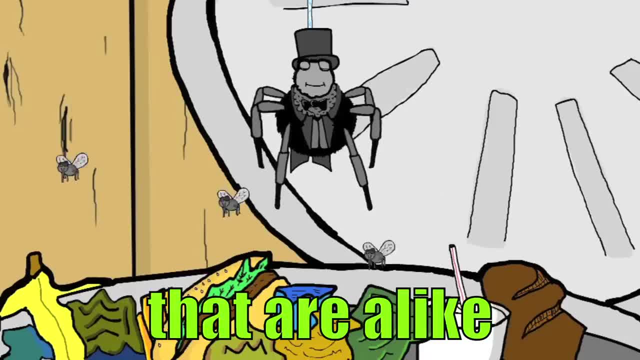 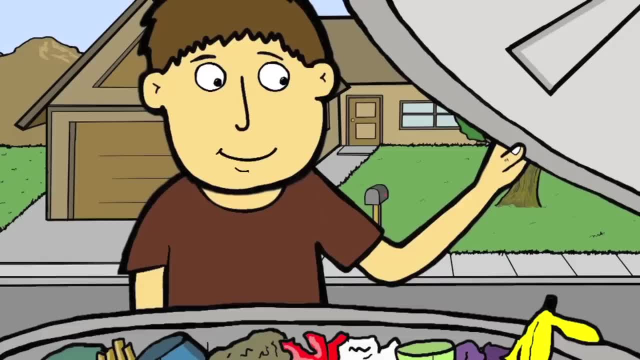 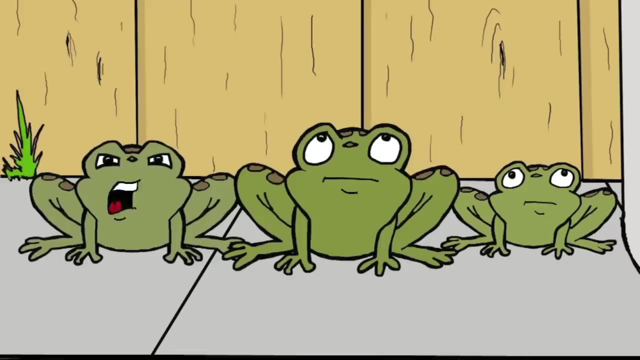 When you do it, Mode's the name, Only the numbers that are alike. Let the others take a hike. Mode is popular. Thanks Toads. Now what can I do for you? Just stay green, Cody boy. Stay green. 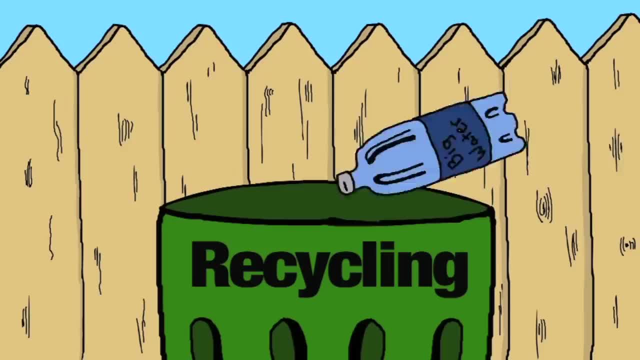 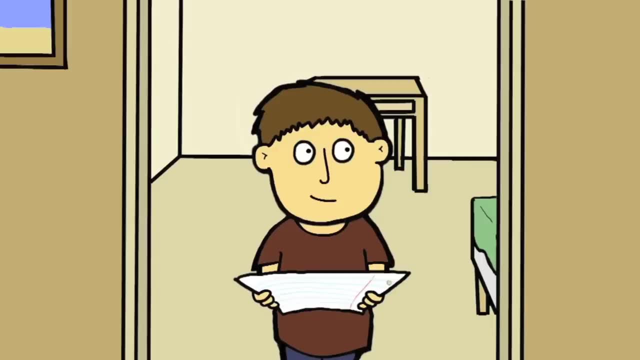 Yeah, yeah, stay green. Okay, Cody, ready for me to help you with your homework. Mom, just relax, I got this, Oh yeah.